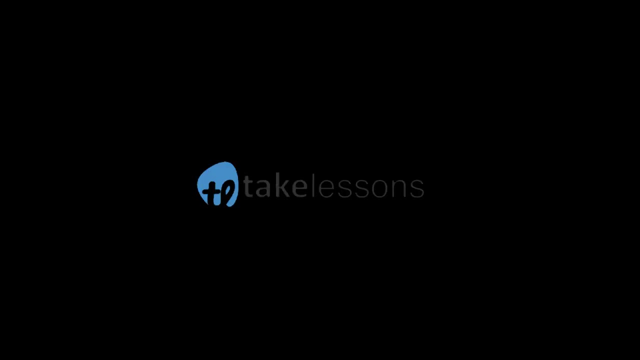 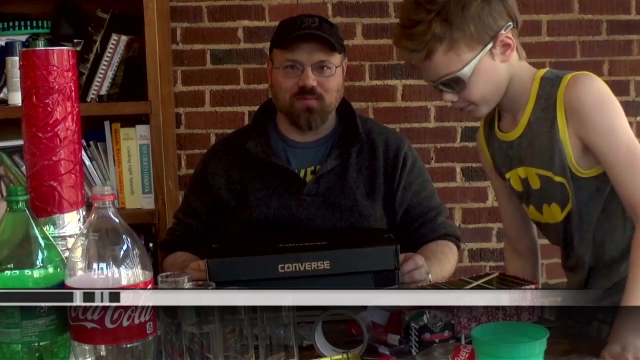 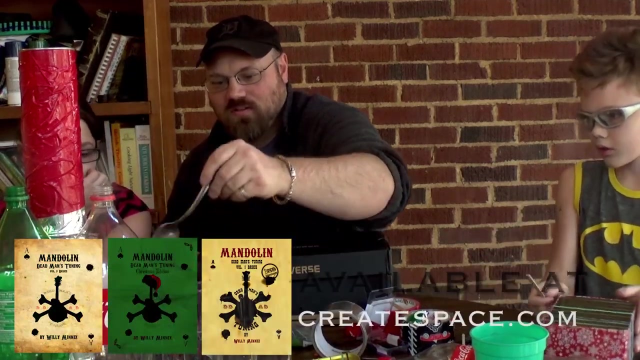 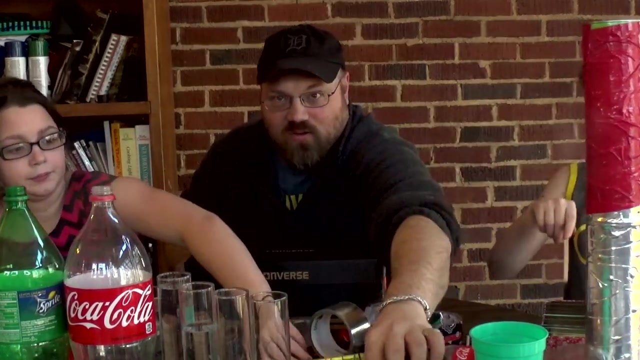 Hi, I'm Willie Medix with TakeItLessonscom. Today we're talking about how to make homemade instruments and in previous videos we've made lots of neat whoops, neat little instruments- Shakers and a rain maker, and we even made a little kalimba. Oh, I'm sorry you keep. 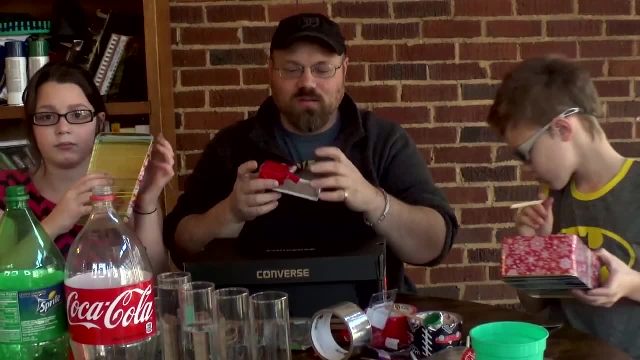 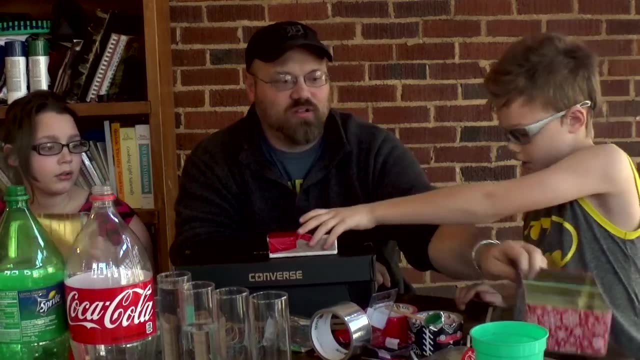 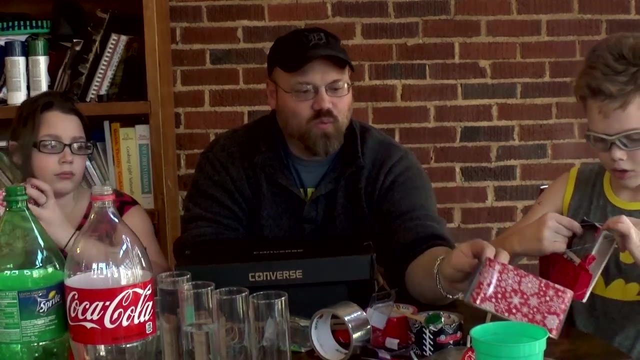 putting that in front of you. We made a little kalimba. Now the kalimba didn't work very well, but it gave me an idea. If we were to combine the little harp boxes that we made a minute ago with the kalimba idea, we might be able to make a neat instrument out of a. 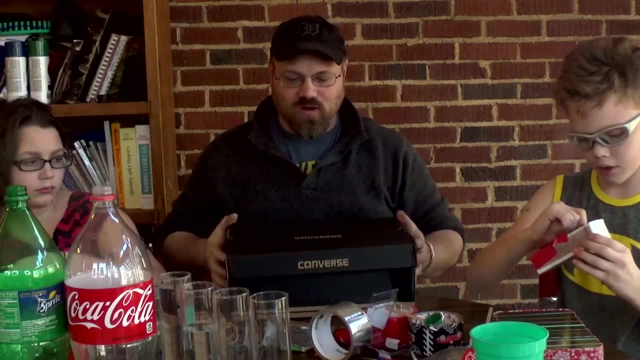 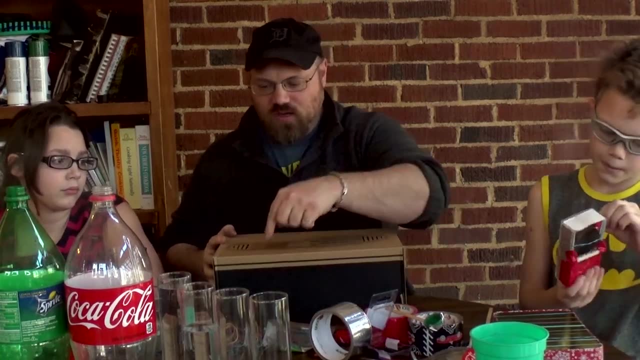 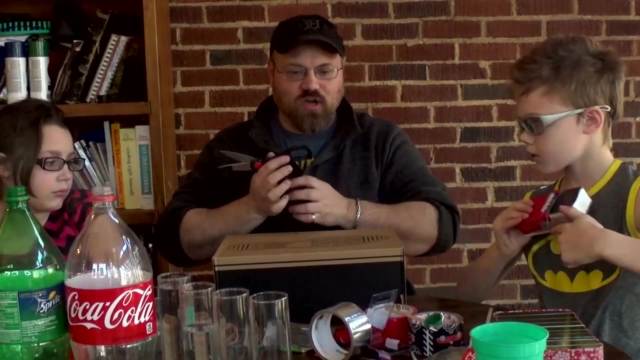 shoe box. So I've got a shoe box here and we're going to turn this into an instrument. right now, What we're going to do is, on the bottom of the box, we're going to cut a sound hole. Now, kids, make sure you have your parents help with this if you're too little, I'm actually 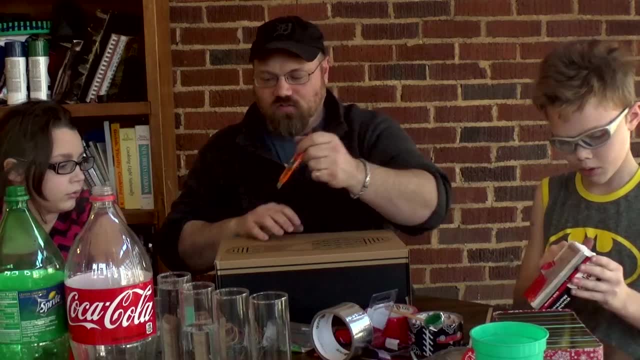 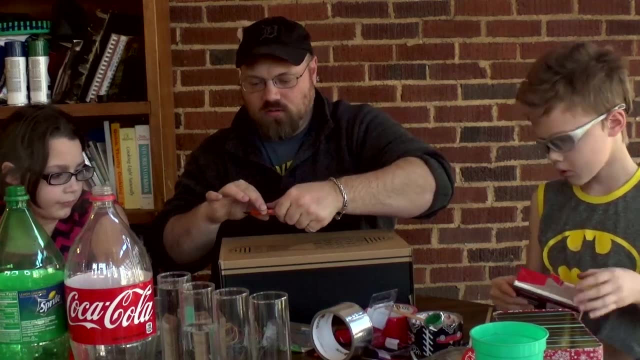 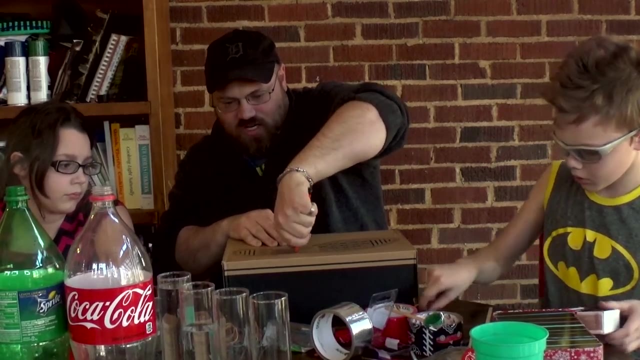 going to use an X-Acto knife and I'm going to be careful with it and I'm going to cut a circle right now. okay, And when I cut this circle, I've got to make sure it's out enough. I'm just going to make as perfect of a circle as I can. 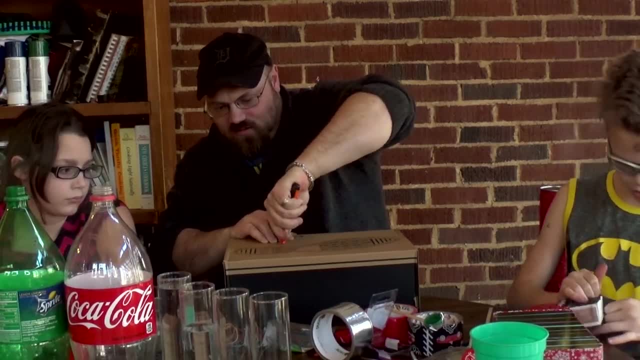 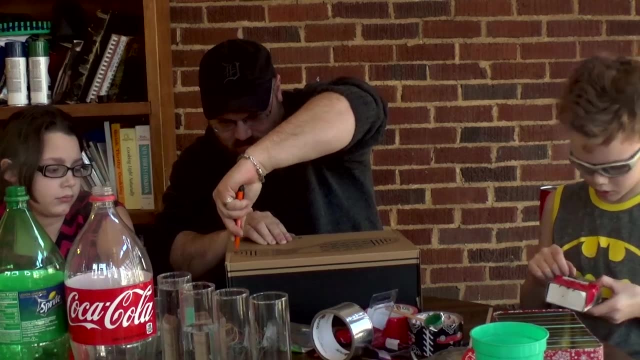 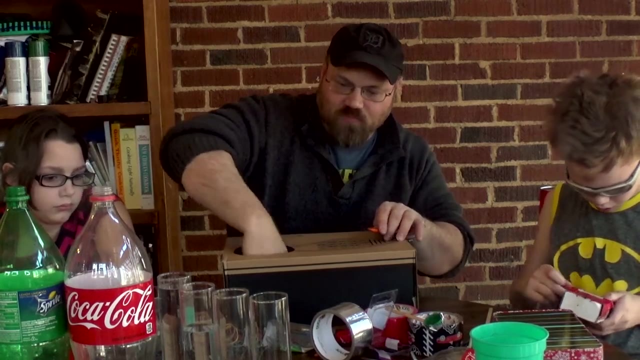 But it doesn't have to be absolutely perfect. You just really need a hole somewhere, because this is going to be the body of the instrument And this instrument is going to be a lot more like a guitar. Now there's my hole right there, And the next thing I need are a couple. 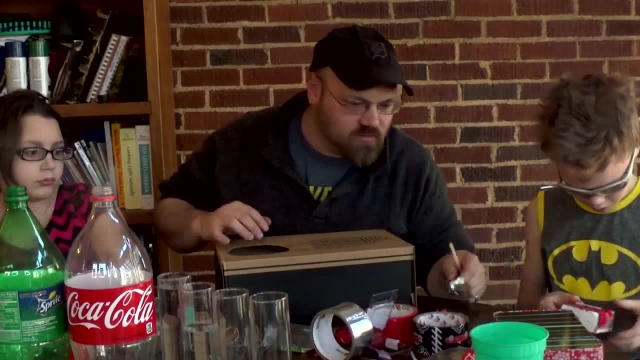 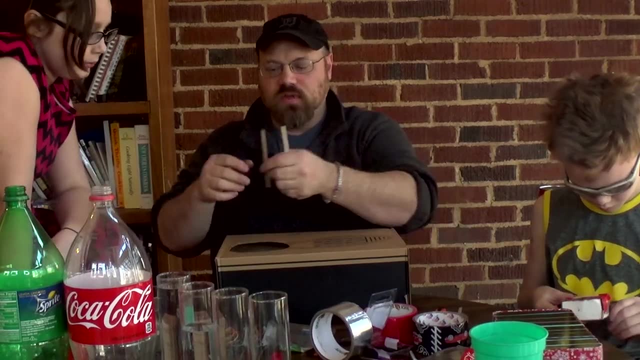 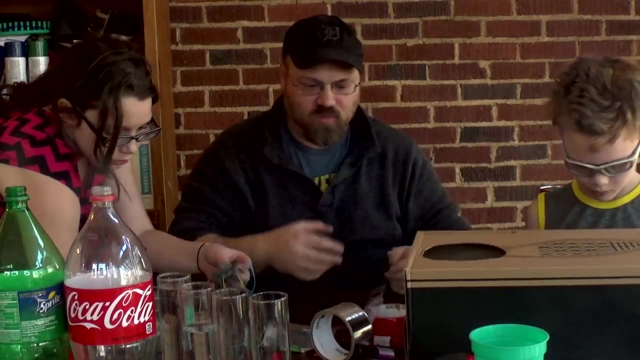 popsicle sticks. These sticks are going to be what hold? I actually want to take this one off here. These sticks are going to be what the strings get held onto, And so I'm going to put this aside for a minute. yep, and we're going to make rubber bands. Now we're going to be. 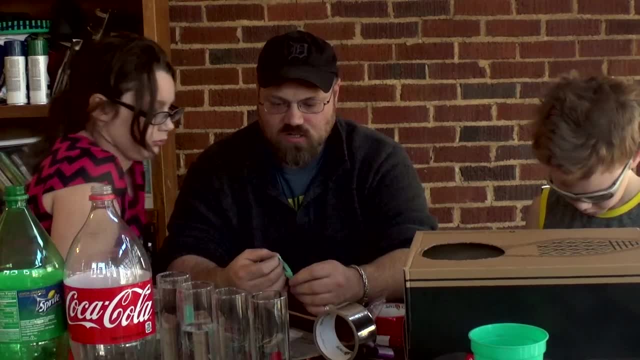 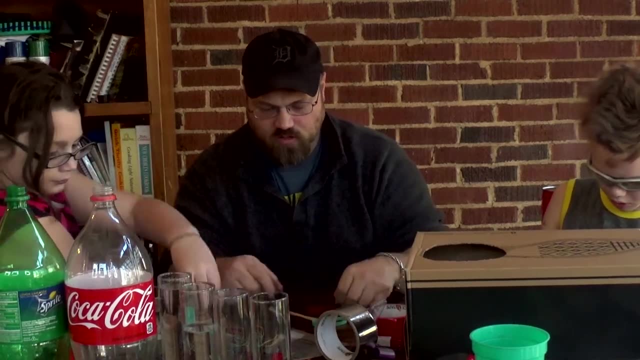 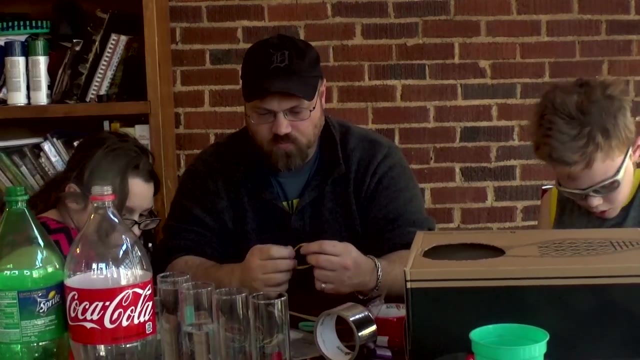 a little more precise than with our harp boxes, and this is going to be a little bit more like the way a guitar works. So we're going to get a thick string and we're going to get a string maybe that's a little bit thinner, you know. Actually, this one's thicker than 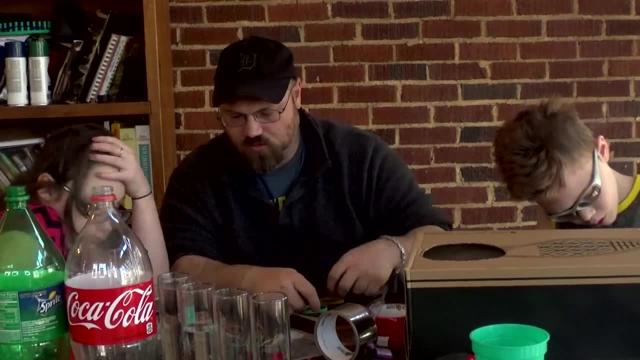 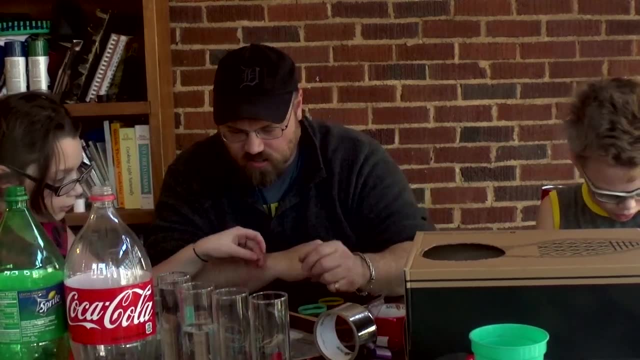 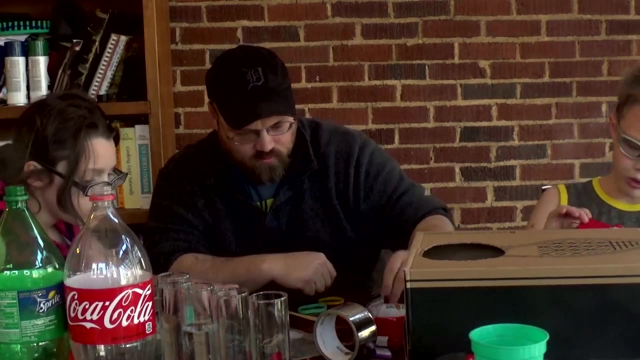 this way, but this one's thicker this way, So we'll try. both of those We'll take. maybe that one's a decent size and this is a good neck size down. Yeah, that would work. We'll put that in there. And then we need some really thin ones. This is pretty thin, And one more. 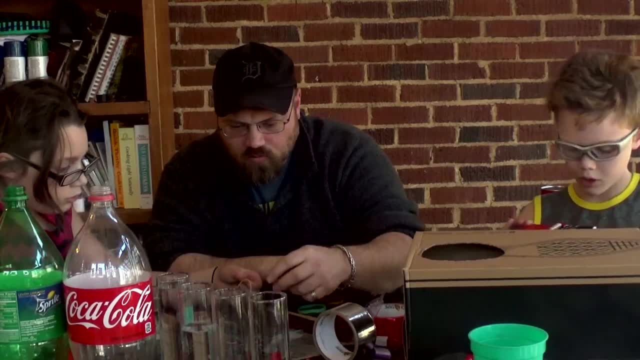 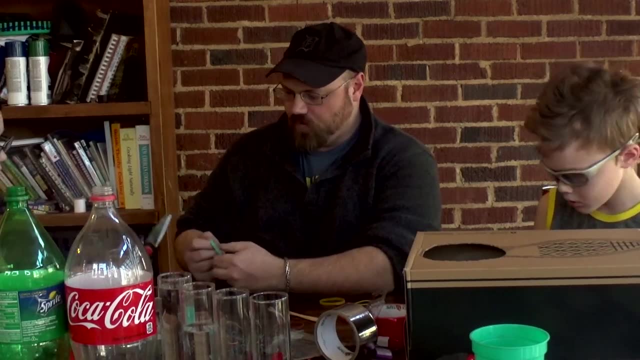 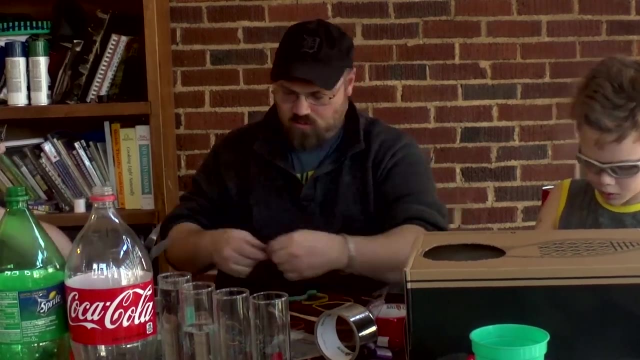 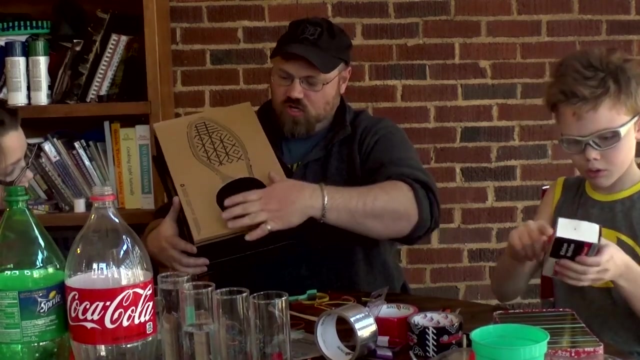 thin one. How about? yeah, that's a pretty good one. Okay, now what we're going to do. Edda, I'm going to hold these. I want you to cut these for me. Okay, there's one Palimbo over here. Now, this little guitar is, we're going to put our strings here and 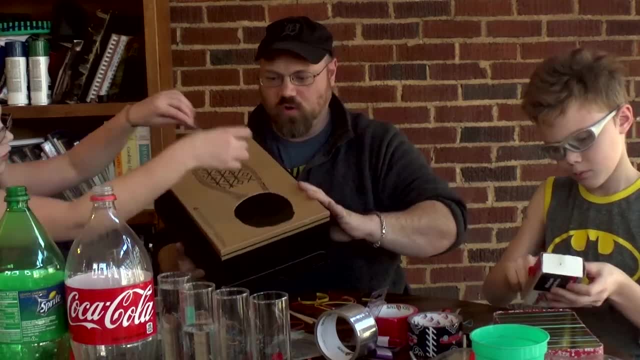 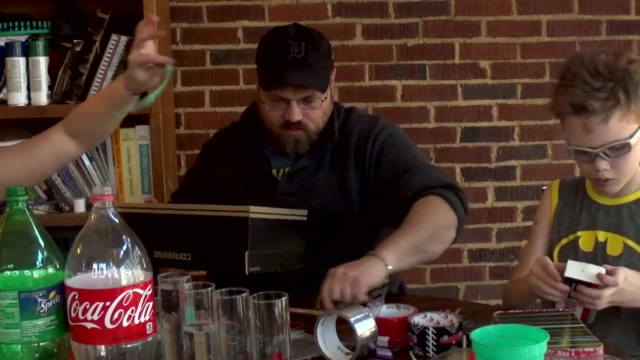 we're going to stretch them across and they're going to come up to here somewhere, So like that. Yep, So now let's make sure that all of our strings will actually stretch that far. This one does. Yeah, you check that one. Okay, let's check these then. 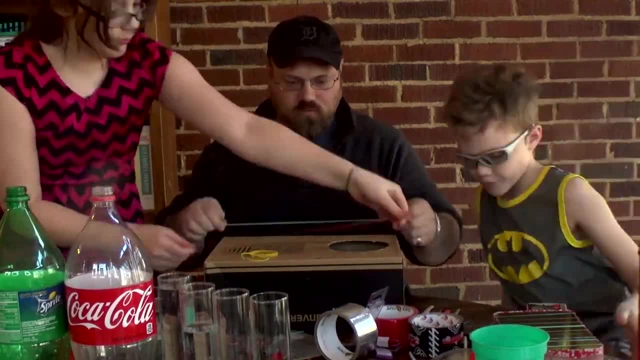 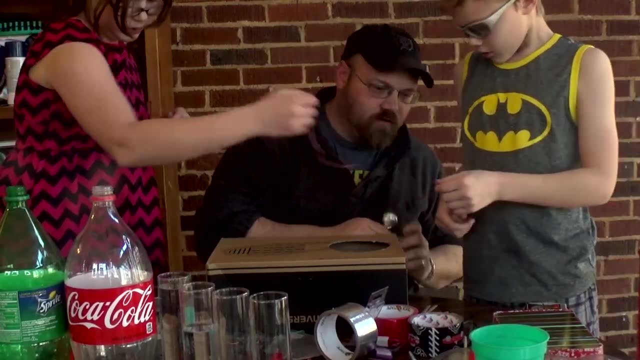 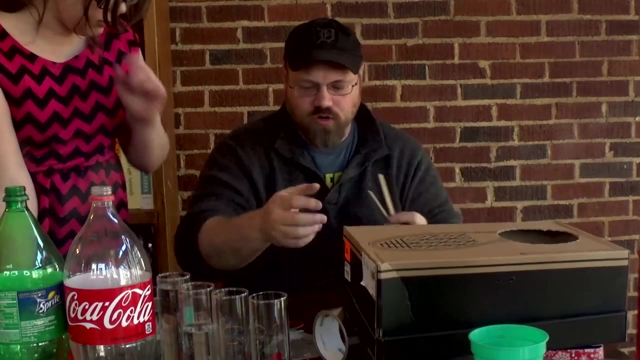 That one does That one will. Now, what we're going to do is we're going to have- can you go in the drawer and see- Okay, the first step we're going to take- our bobby sticks or craft sticks. 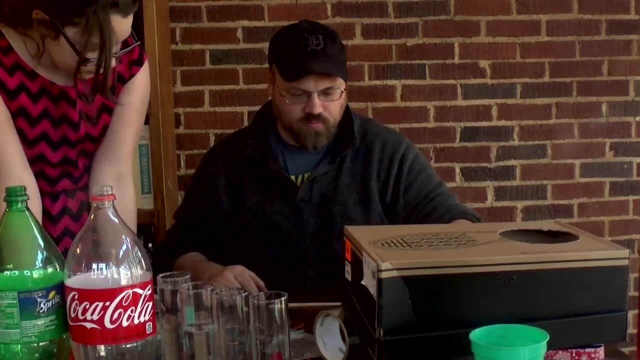 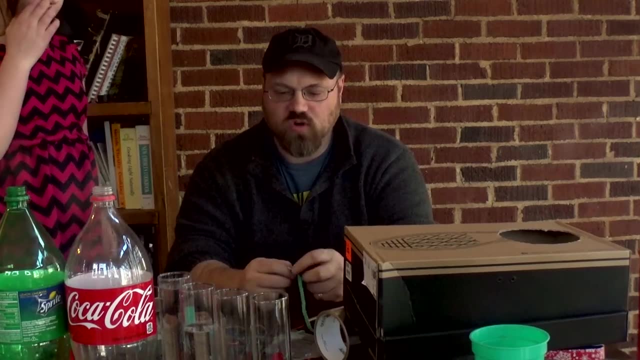 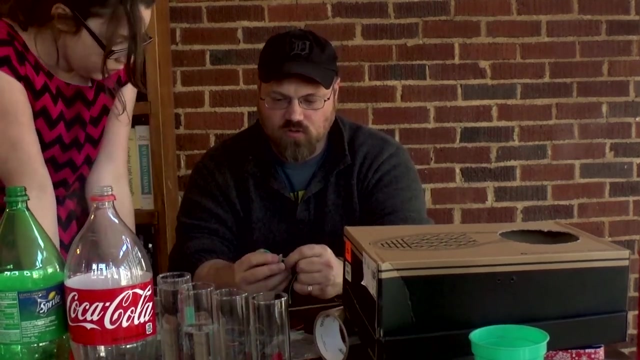 and we're going to start putting our rubber bands on it. Now, you could glue these on if you wanted to. Okay, Maybe with rubber cement, but I'm just going to tie them on right now. Just take it and tie it up. No, I've got to do it in order. So what you want to do is you're going to 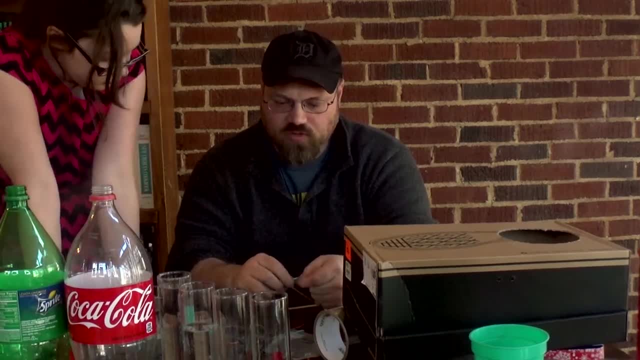 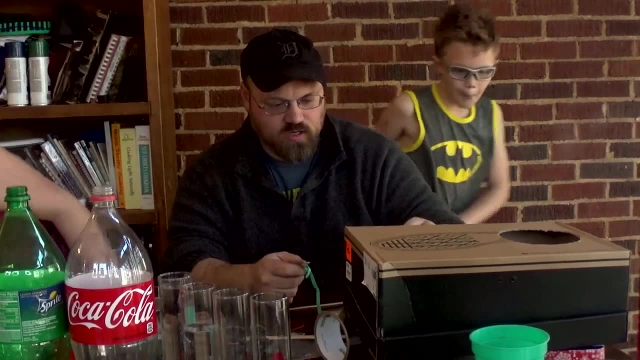 tie your sticks in order, starting with your thickest rubber band- Thanks buddy- And going all the way down to the thinnest one. Okay, So there's one and here's another. You know how a guitar has thick strings. 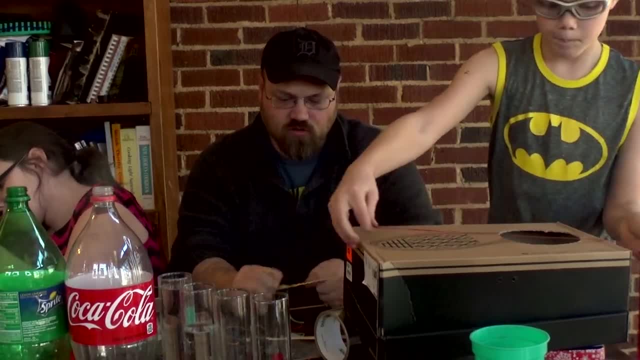 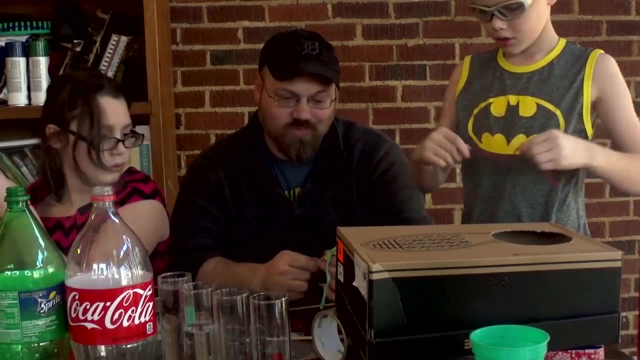 Yeah, Thin strings on one end and thin strings on the other right. This is how. this is kind of what we're doing here. Tune it. Yeah, so you can tune it Now. I don't know if we'll be able to tune it. 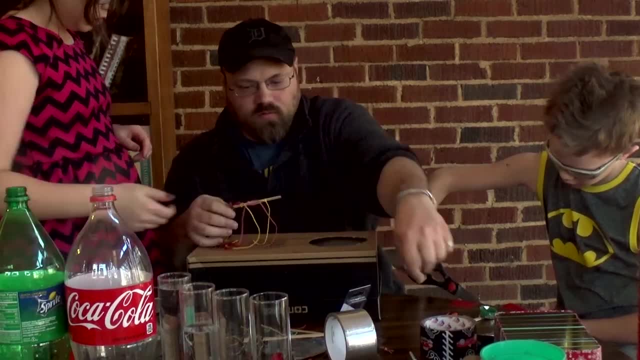 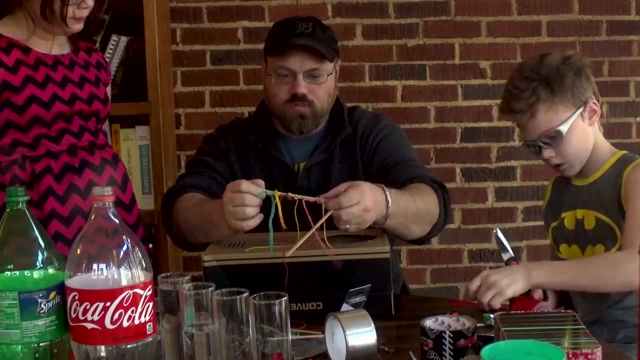 Okay, you got that. Maybe you should put some on the rack. Well, it won't matter, because what we're getting ready to do is we're going to sandwich them right here onto this piece of wood. What we're going to do is we're going to tape. 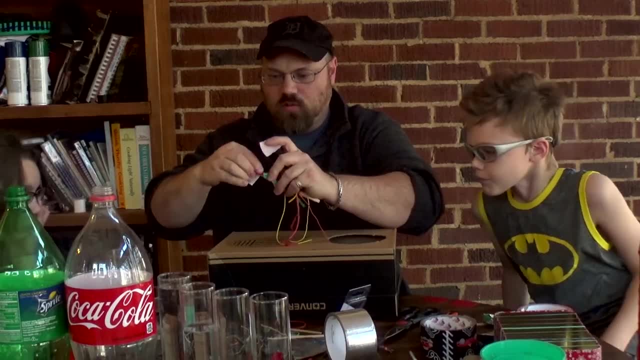 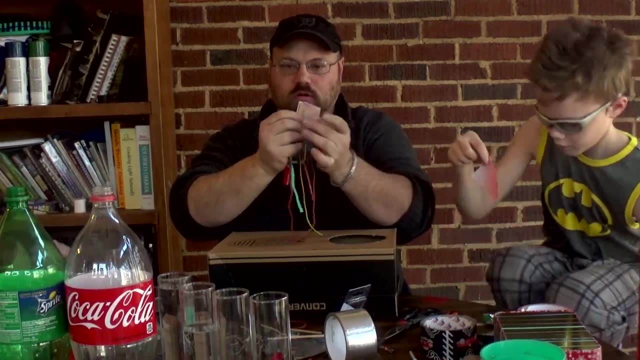 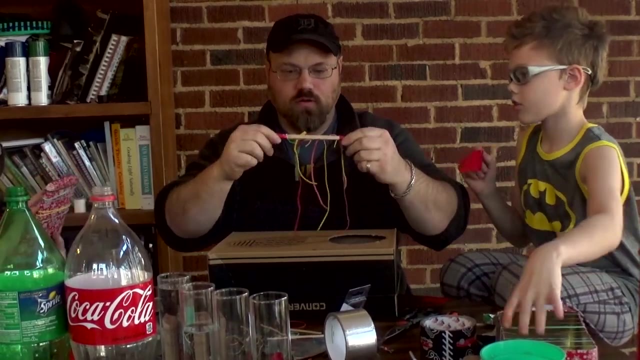 the ends. It's all right, We might need it for something else. I'm going to tape this side right here. I love these harp thingies. They're fun. huh, They're so cool. Okay, And then we're going to take this thing that we just made and we're going to tape it on. 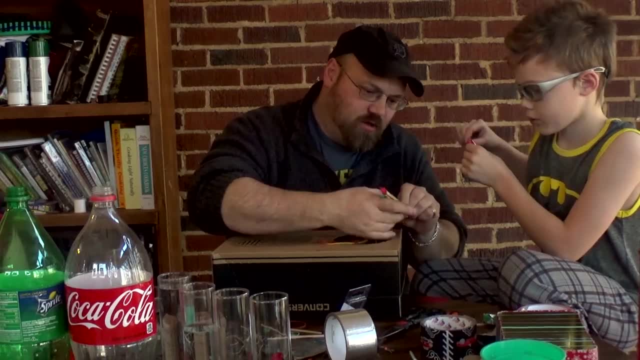 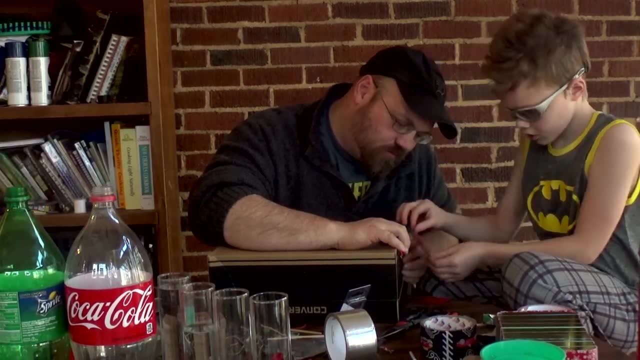 here, Okay, And then we're going to tape this thing that we just made and we're going to tape it to the end of our guitar. Now, wait a minute. How we're going to do this is we're going to tape one end over here. Hopefully they can see that. 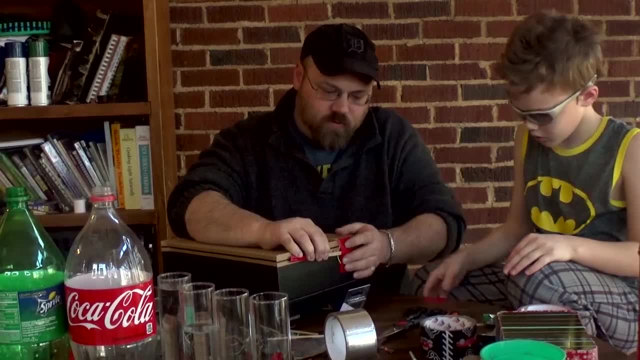 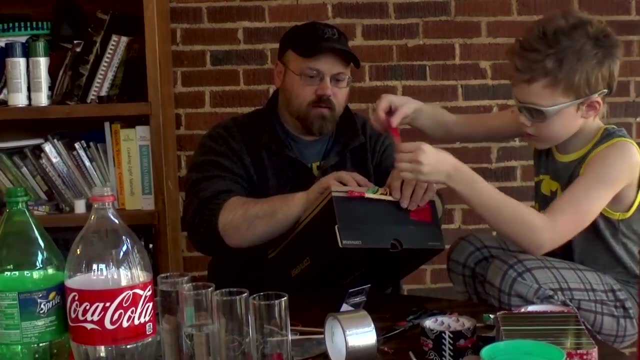 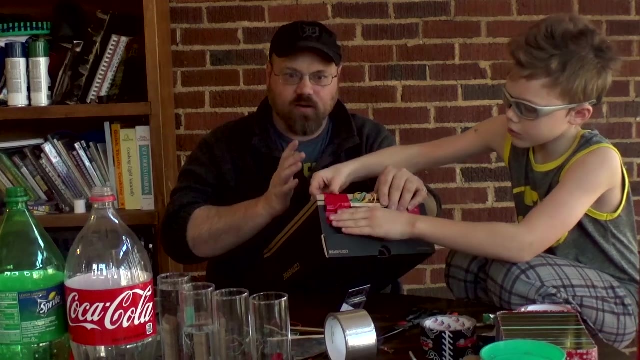 One end. what may I zoom in? No, no, it doesn't need to zoom in like that And one end on the other side, like that. Now, every instrument has to have a base, It has to have a bridge or a saddle that the strings go over. I mean every stringed. 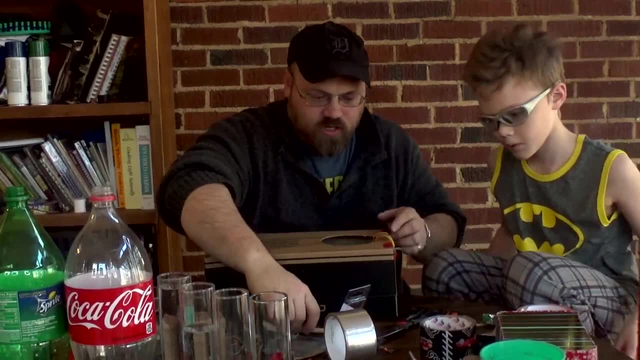 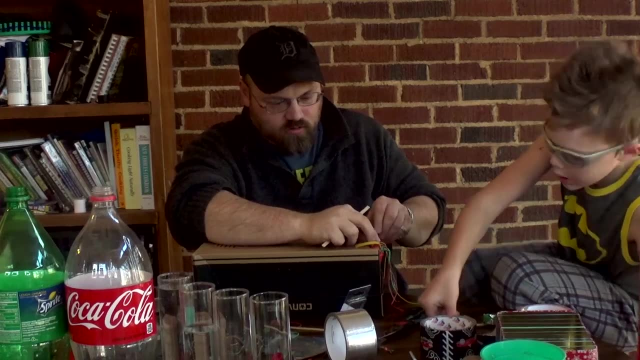 instrument And it has to have a nut that the strings go on on the other end. So what we need to do for our bridge is we need to put a piece of wood over here so that it lifts it up off the soundboard a little bit, And this wood's kind of thin, so I'm going to 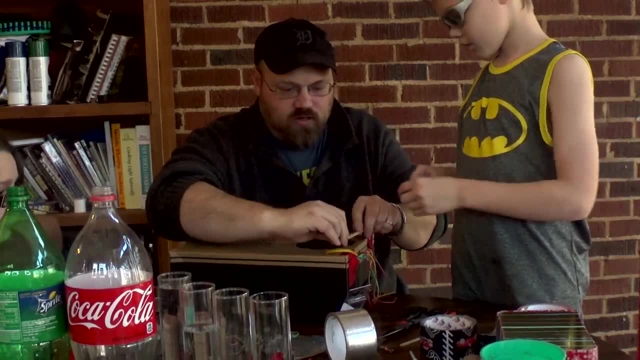 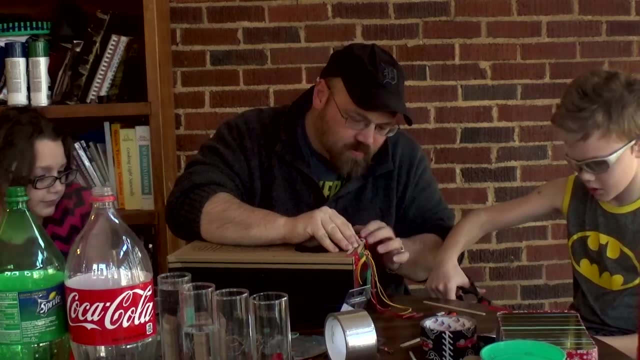 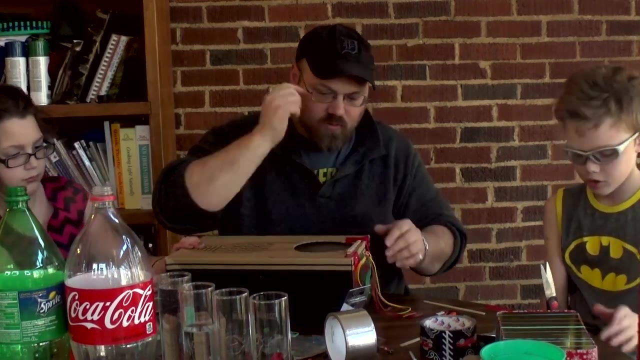 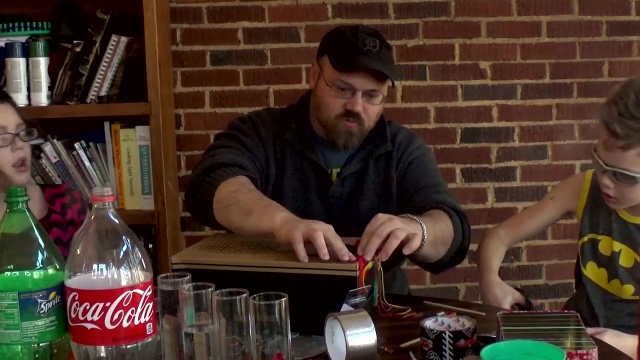 take two pieces and put it together. And, Gideon, can you cut us a piece of tape, a couple pieces of tape, so we can tape these on now and right here on this side, And then we're going to do the exact same thing on the other side, Just like this. Now, this is where it gets. 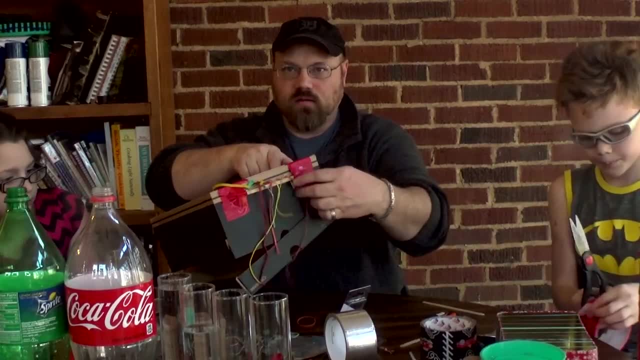 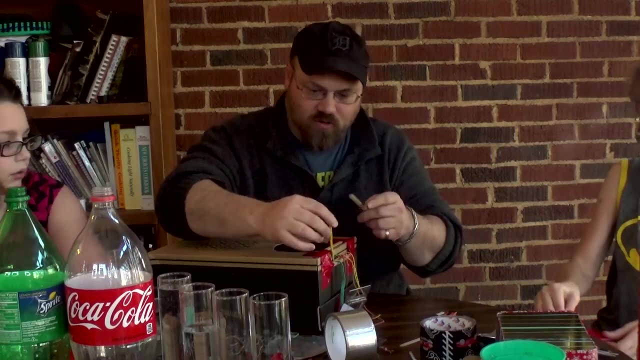 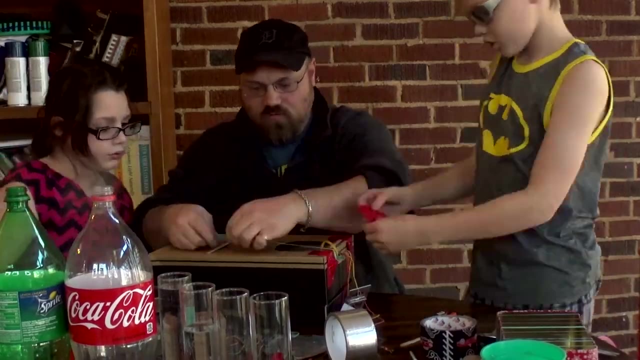 to be kind of fun. The other end of the string has to be tied onto this part of the string. The other end of the string has to be tied onto this part of the guitar Which you're going to stretch down here. Yeah, but I don't.